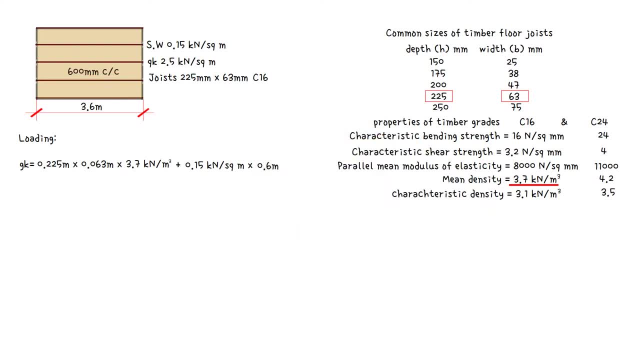 multiplied by joist spacing of 0.6 meters, This corresponds to a value of 0.09 kilonewtons per meter. The imposed load equals the value of the floor joist. The characteristic imposed floor load of 2.5 kilonewtons per square meter multiplied by 0.6. 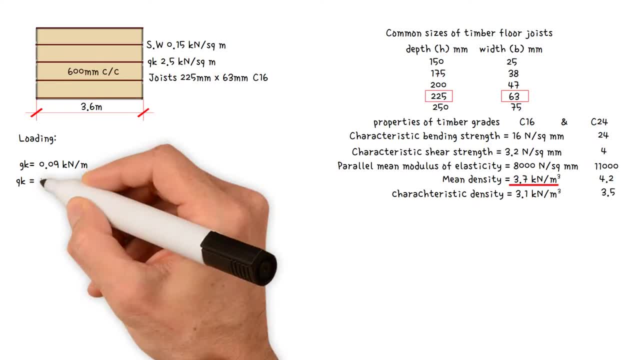 meters joist spacing. This gives a value of 1.5 kilonewtons per meter. We'll need both the ultimate limit state and the serviceability limit state to figure out the stresses and deflection In the serviceability limit state. uniformly distributed load equals total unfactored loads. 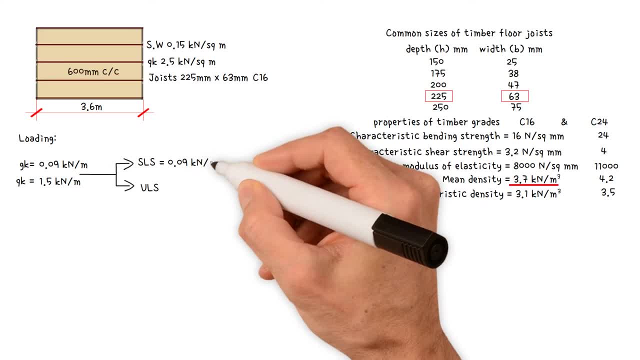 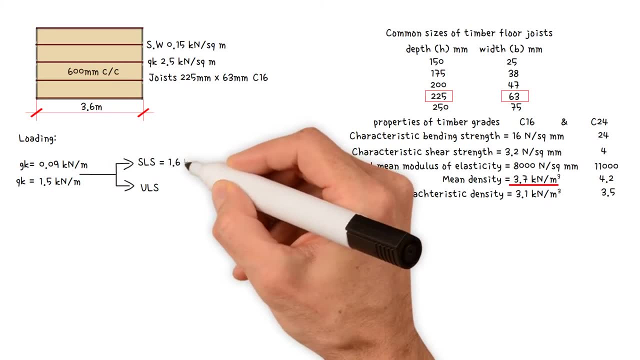 which equals dead load, 0.09 kilonewtons per square meter. This gives a value of 1.6 kilonewtons per meter. Uniformly distributed load in ultimate limit state equals total factored loads, which equals dead load 1.35 times 0.09 kilonewtons per meter. 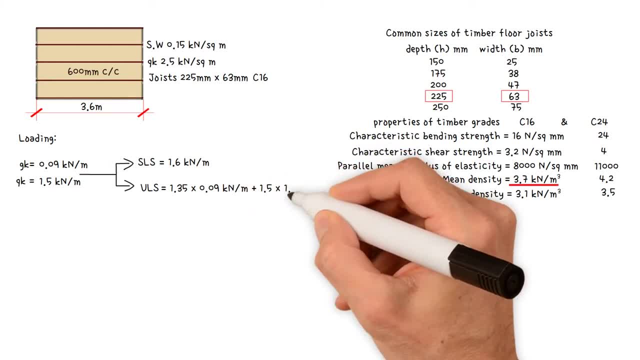 plus imposed load 1.5 times 1.5 kilonewtons per meter. This results in a value of 2.4 kilonewtons per meter. We should now be able to calculate the applied design forces. The bending moment of a simply supported beam is equal to the design load of 2.4 kilonewtons per. 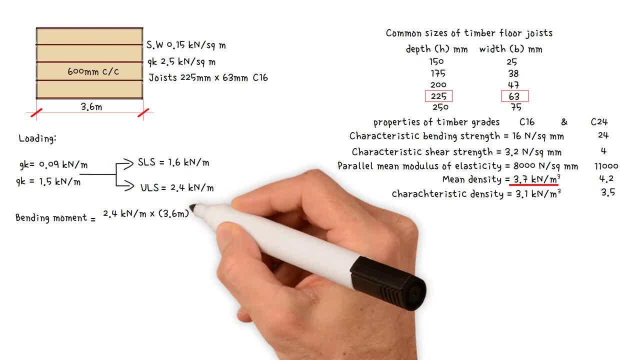 meter multiplied by the span of 3.6 meters squared divided by 8. This results in a value of 3.85 kilonewtons meter. The shear force for a simply supported beam is equal to the design load of 2.4. 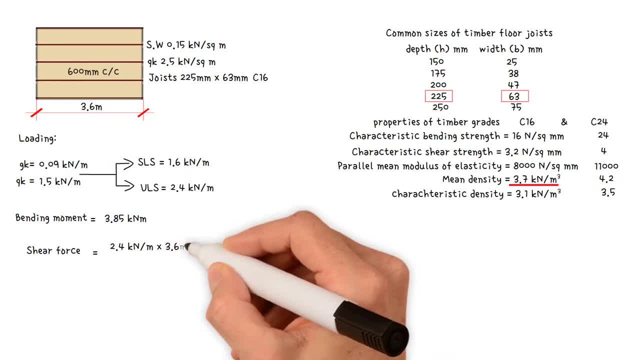 kilonewtons per meter multiplied by the span of 3.6 meters. divided by 2. This gives us a value of 4.3 kilonewtons. The applied bending stress equals the design bending moment divided by the elastic modulus of the joist, which is calculated as the width times the depth of the section squared. 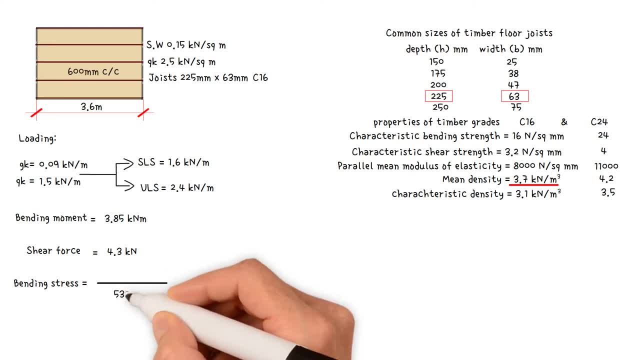 divided by 6, giving us a value of 532 times 10 to 3 millimeters cubed. To convert kilonewton meter to newton millimeter, the bending stress equals the design bending moment 3.85 times 10 to 6, divided by the elastic modulus 532 times 10 to 3.. This results in a value 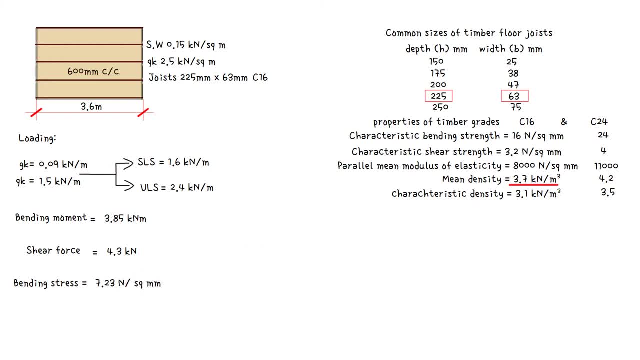 of 7.23 newton per square millimeter. This value must be compared to joist strength. Timber is a hygroscopic material that absorbs and releases moisture, depending on the amount of moisture in its surrounding environment, Because the strength and stiffness properties. 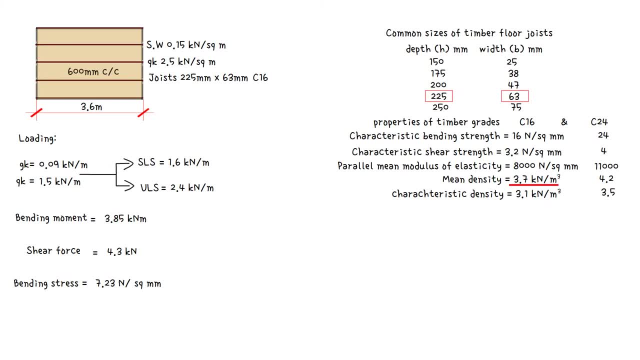 of timber are affected by moisture content, the environment around the timber must be considered. There are three types of services. The following are examples of typical environments and the corresponding service class. Service class 1: intermediate floors- warm roofs. internal and party timber frame walls. Service class 2: ground floors- cold roofs. 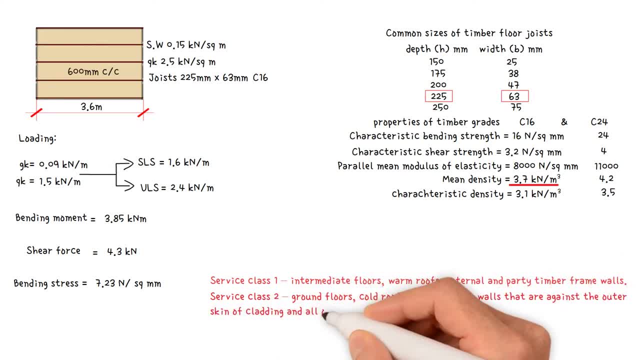 timber frame walls that are against the outer skin of cladding and all other instances where the timber is protected from direct exposure to water, Service class 3, external, fully exposed. The strength of a piece of timber is proportional to the duration of the load. 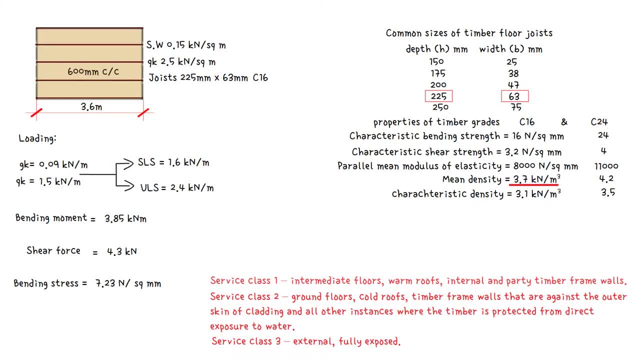 The greater the duration of the load, the greater the strength of timber required to resist that load. To that end, a variety of factors are applied to the characteristic properties of the timber: The values for the factor KMOD, which is applied to the strength of the timber and is based on the 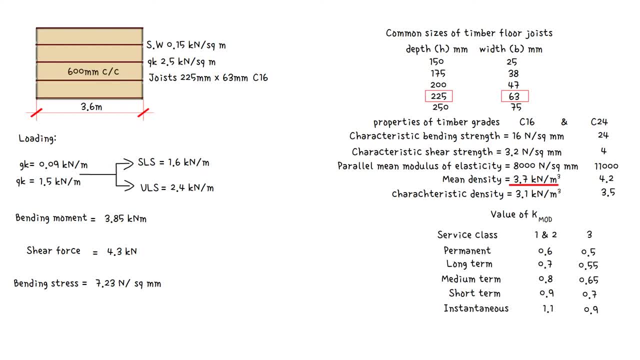 imposed load duration are provided in the table below. The imposed floor load with the self-weight of the joists and superimposed dead load is a typical critical condition for timber floor joists within a building. This load condition results in a value of KMOD of 0.8 because it is 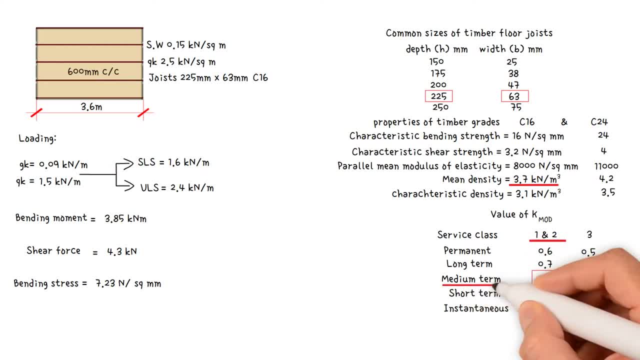 subject to an imposed load, which is defined as medium term, as well as superimposed dead load. Design bending strength equals this formula. KH is modification factor. If a member is less than or equal to 150 millimeters deep and has a material density of less than 7 kilonewtons per meter cubed, the factor is defined. 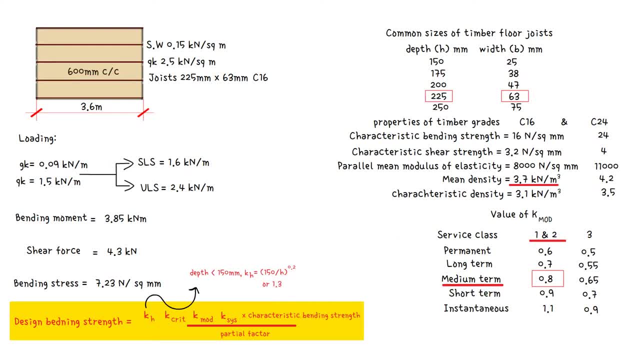 as or 1.3, whichever is the lesser. For all members that are greater than 150 millimeters deep, the value of KH is taken to be 1.. This factor is applied to the bending capacity of the joist if the compression face of the floor 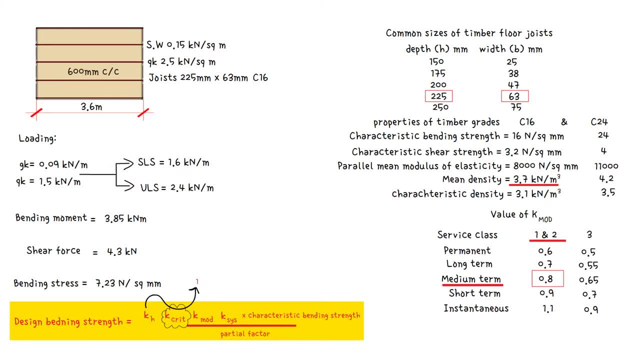 joists is not restrained against bending induced torsional rotation, which is a rare condition. In most cases, there is no risk of lateral torsional buckling affecting a floor joist. This is due to the presence of a floor finish that acts as a restraint on the joists. 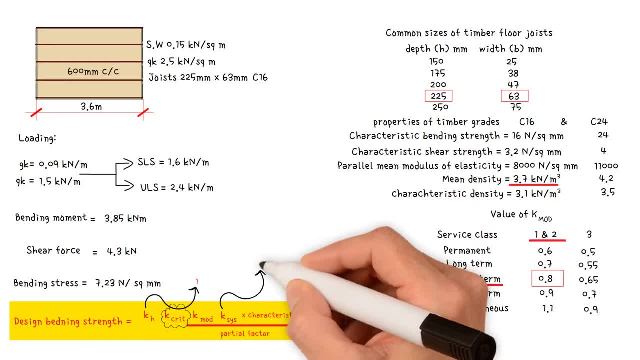 This load sharing modification factor, which equals 1.. Characteristic bending strength, which equals 16 Newton square millimeter for C16.. The partial factor has a value of 1.3.. Therefore, the design bending strength equals 1 times 0.8 times 16, divided by 1.3, which gives us: 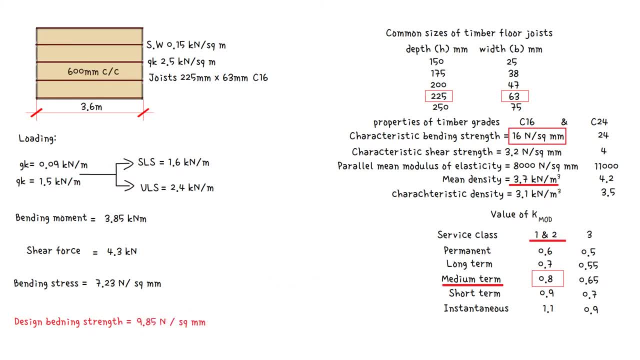 a value of 9.85 Newton per square millimeter, which is greater than 7.32 Newton square millimeter. Furthermore, we must check the shear resistance of the joists For a certain group of joists. we must check the shear resistance of the joists. 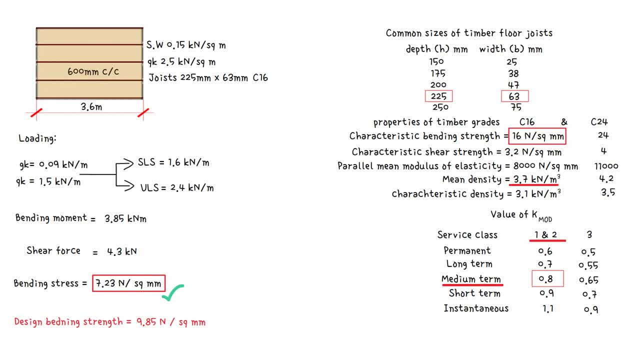 Simply supported joist, the design maximum shear force is equal to the design reaction. In the case of timber, the maximum design shear stress, not average shear stress, needs to be checked against the design shear resistance. The maximum design shear stress of a rectangular section is calculated using 1.5 times the design applied shear force divided by the depth and the width of the section. 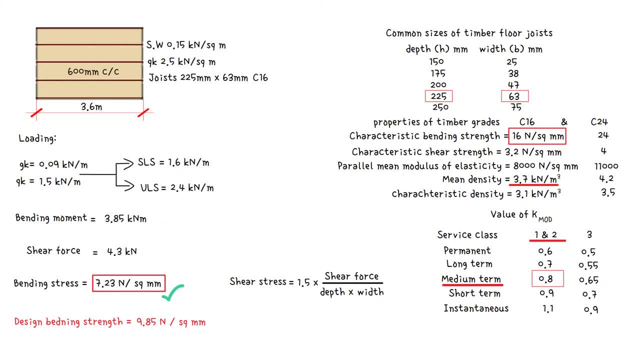 In order to take into account cracking within the timber, the width of the joist is reduced by factor of 0.67.. As a result, applied shear stress equals 1.5 times the design applied shear force multiplied by 4.3, times 1000 to convert to Newton. divided by joist depth: 225 mm. divided by width: 63 mm. multiplied by factor 0.67.. 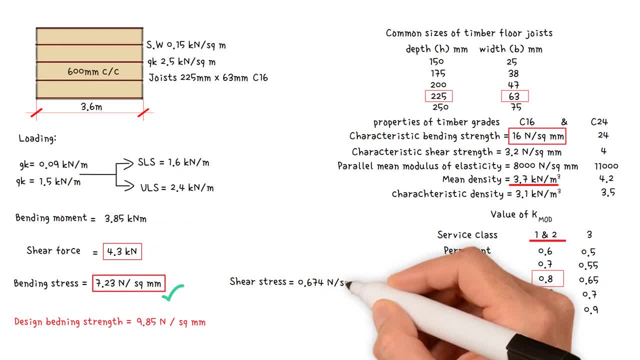 This results in a value of 0.674 Newton per square millimeter. This formula equals the allowable shear stress, That is, 0.8 times 1 times 3.2, divided by 1.3.. This gives us a value of 2 Newton per square millimeter, which is greater than the value of 0.674 Newton per square millimeter. 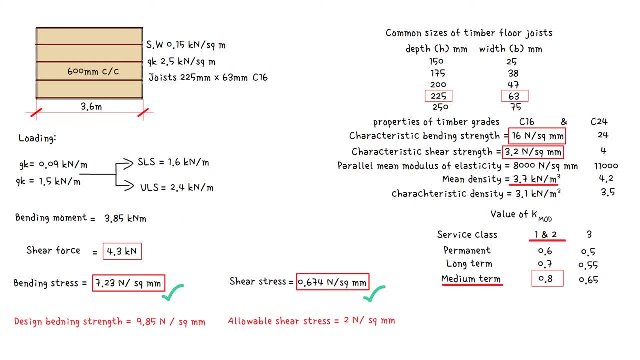 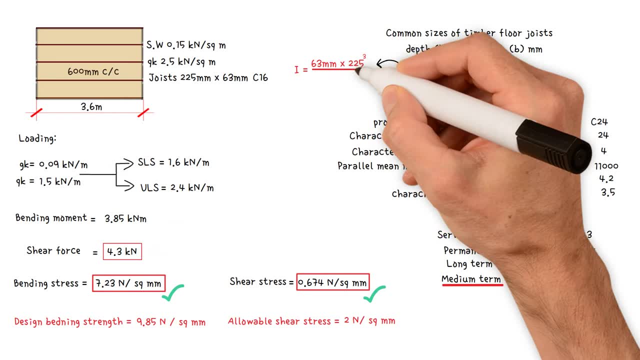 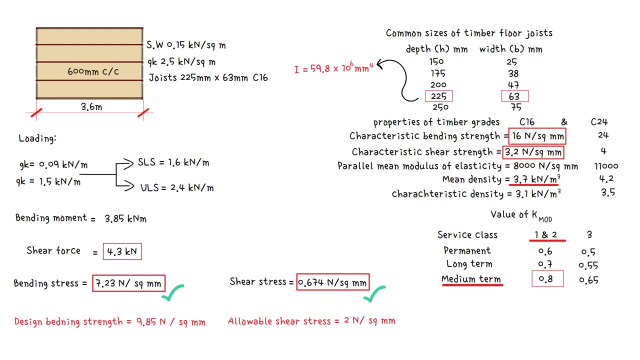 Finally, we must to undertake deflection check. The moment of acceleration Inertia of the section equals width, 63 mm times depth, 225 to 3 divided by 12. This gives us a value of 59.8, times 10 to 6 mm to 4.. 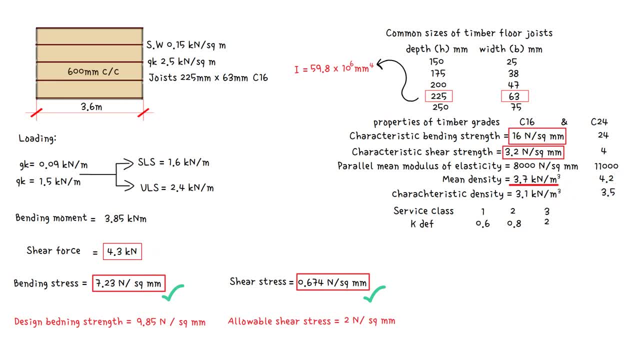 Deformation factor for service class 2 equals 0.8.. C16 has a parallel mean modulus of elasticity of 8000 Newton per square millimeter. So first we need to work out deflection due to dead loads. This gives us a value of 0.74 mm divided by the moment of inertia of 59.8, times 10 to 6, times 1, plus deformation factor 0.8.. 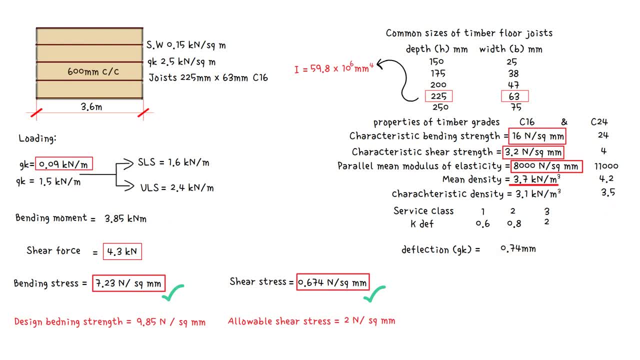 This gives us a value of 0.74 mm. The deflection due to imposed loads, including a mover, equalson times depth 223 to". divided by distance, 0.2, times deflection due to imposed loads, including floor due to lean, tenemos 5 x. 1.5 kNm per meter times joist span: 3600 to 4, divided by 384,. divided by parallel mean modulus of elasticity: 8000, divided by moment of inertia: 59.8, times 10 to 6, times 1, plus deformation factor, 0.8, times 0.kNm3.. 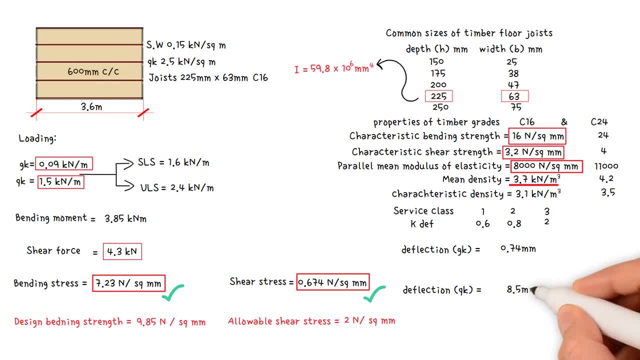 0.3,. this gives us a value of 8.5 mm. The sum of these deflections provides the overall deflection due to bending. However, there is the issue of deflection due to shear. This is rarely a critical condition, but it is prudent to add 10% to the overall deflection to arrive at a final value.